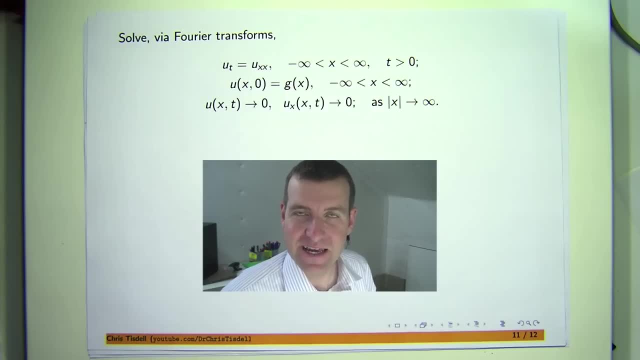 Hi again everyone. Chris Tisdell here again. In this presentation I'm going to continue my series of videos on Fourier transforms and their applications to partial differential equations And in particular I'm going to solve the following problem via the method of Fourier transforms: So we've got a partial differential equation here You might represent. 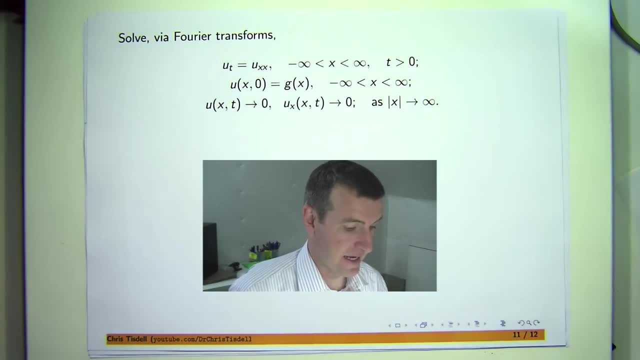 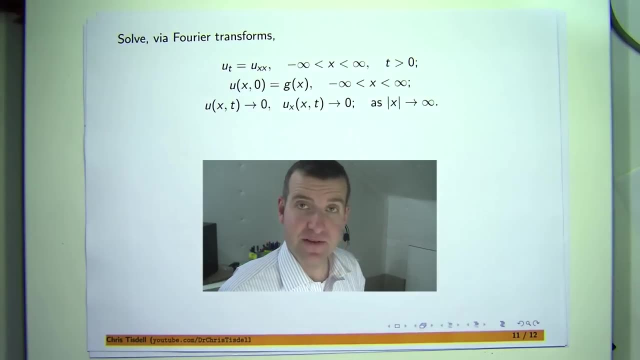 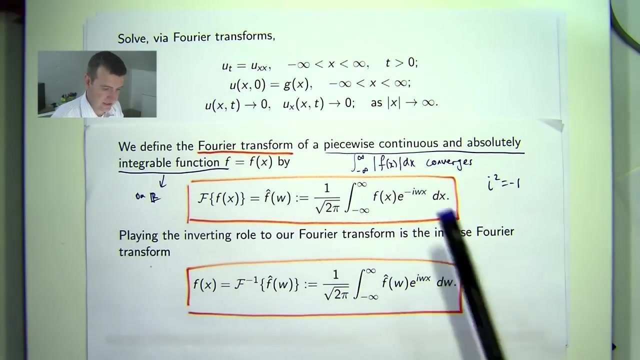 the temperature at position x and time t in some infinitely long bar. You've got some initial temperature and some limiting conditions. Now in previous videos we defined the Fourier transform of a function. it's an integral transform and its inverse which kind of? 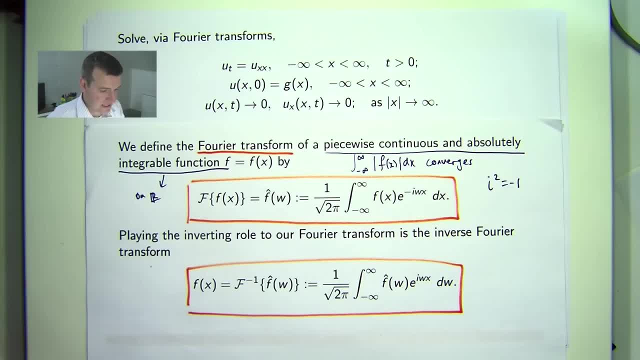 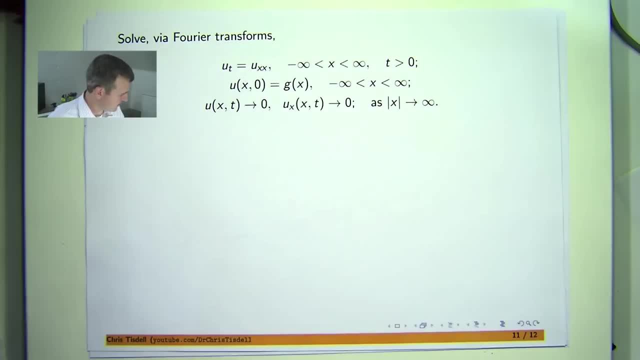 undoes the Fourier transform. Now, the particular interest in these kinds of transforms is in their application to differential equations and their solutions. Now we're going to use two important concepts to solve this particular problem. First of all, we are going to use transform of derivatives, and I talked about that in a previous video. 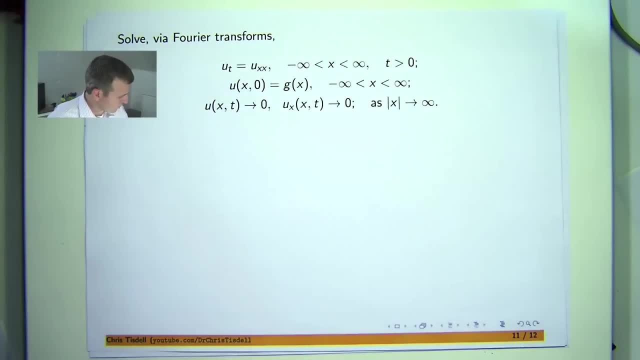 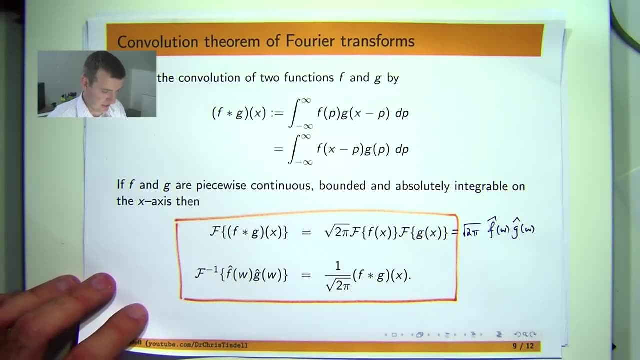 So here are some transform of derivatives And we're also going to use the so-called convolution theorem of Fourier transforms. You define the convolution of two derivatives. You define the convolution of two functions, f and g, to be this sort of improper integral with a shift in one of the functions. And then let's say you wanted to take the inverse. 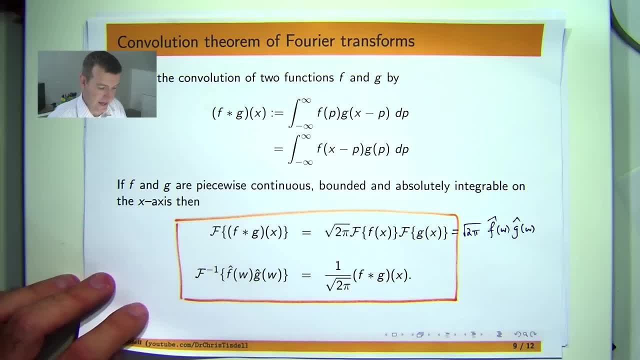 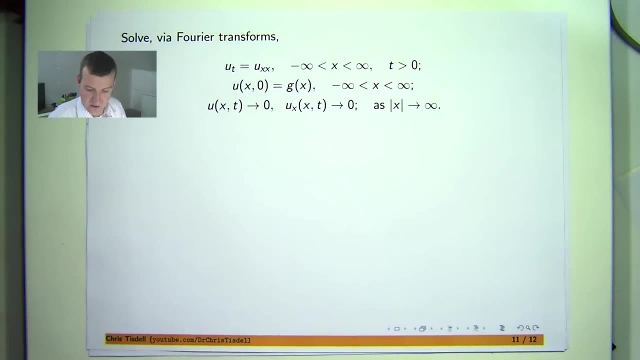 transform of a product of Fourier transforms, then it's just basically this: constant times, the convolution of the two functions, And again there's another video on that as well. So the interest in or the interesting part of this video is the solution or the application. 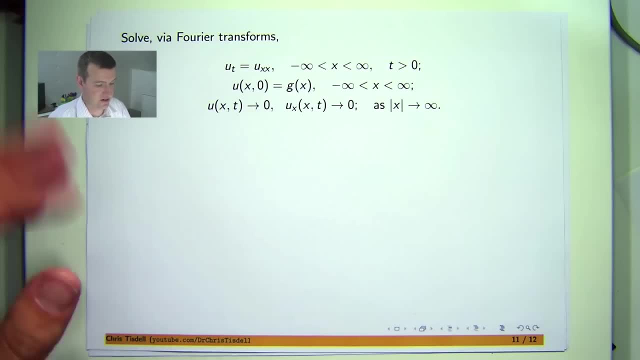 of Idee, of the previous ideas to this kind of problem. Okay, so let's get down to it. Okay, the idea with any kind of transform method applied to a problem involving differential equations is the following: You transform the PDE to some new setting. Hopefully the problem in the new setting is. 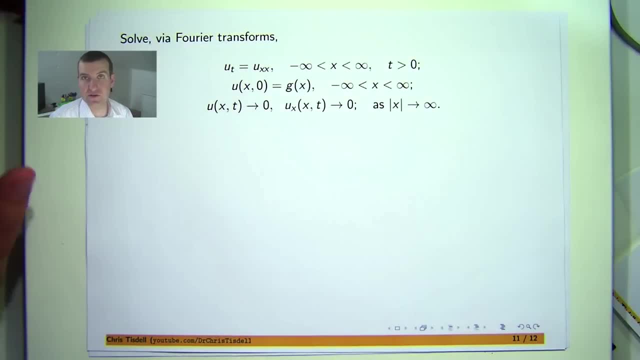 simpler than the original one. This is under 2D indication. You transform the PDE to some new setting. Hopefully the problem in the new setting is simpler than the original oneное that this is a might not mean it's simple, then how would you like me to simplify it by myself, as I call the video? 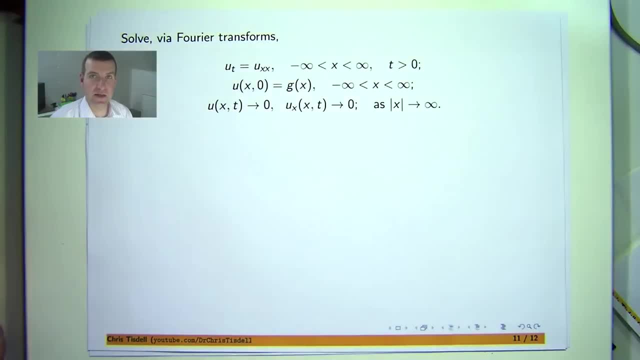 You solve the DC maing. it's 0.. s to Liter and f or f and or s from 0 to f or x or f and g to f or v and d to f and g to f and g to f or p and g. personne. 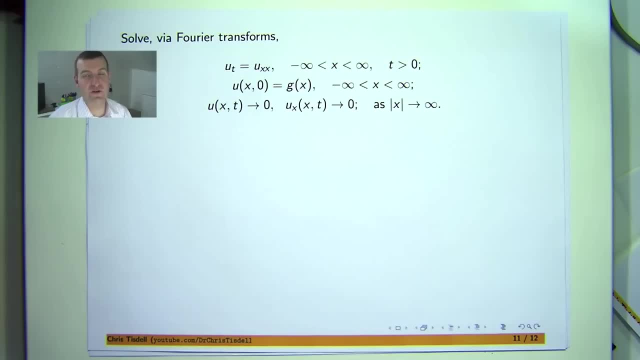 the original one, You solve the transform problem And then, to recover the solution to the original problem, you untransform or inverse, transform everything. So the method is best explained or best understood via example. So let me show you an example, I'm just going. 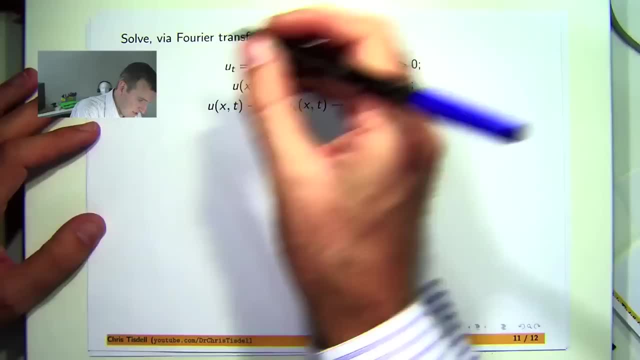 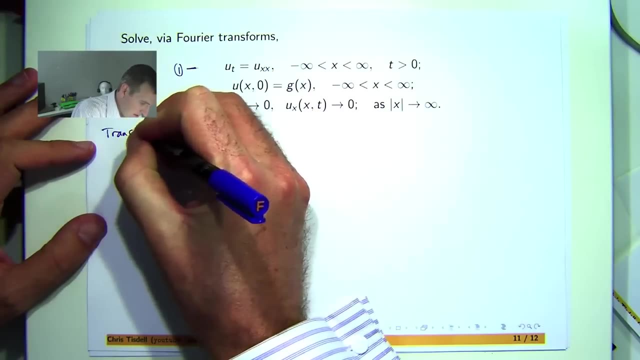 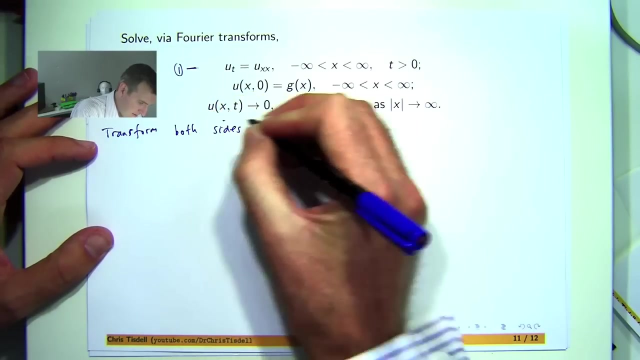 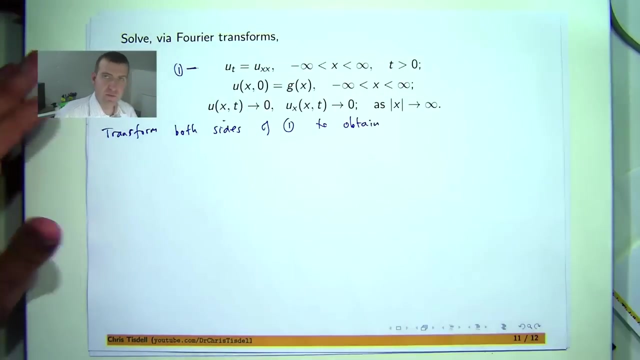 to work through this step by step. So let's call this, say 1.. So we transform both sides of 1 to obtain the following. Now remember, when we take the plus transforms, we're essentially transforming with respect to the spatial variable. 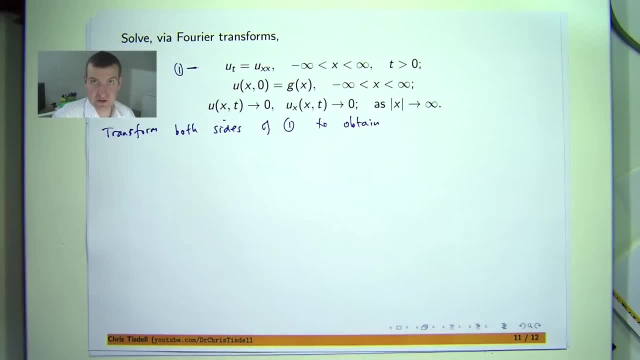 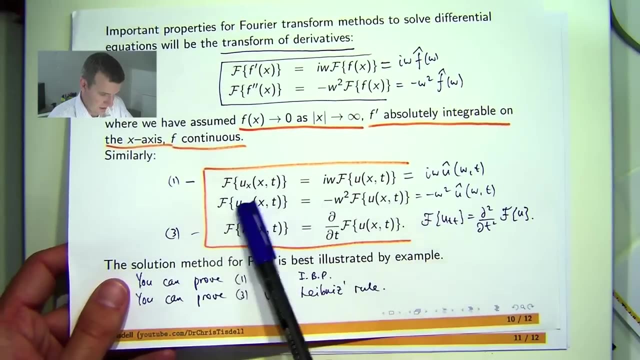 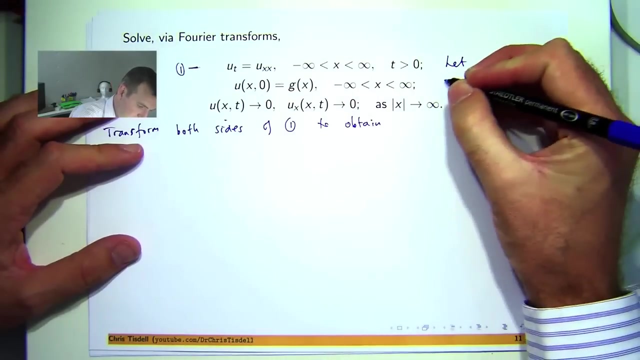 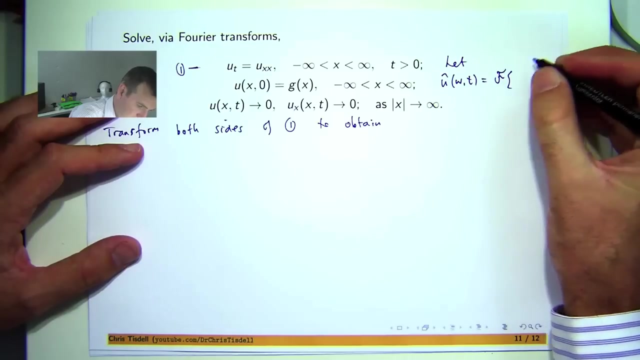 Now for the t variable. this derivative will just be the derivative of the transform, And this one can be written down from this middle line here. OK, So I'm going to let a little bit of notation. let u of w, t be the Fourier transform of u with respect to the x variable. So this would be: 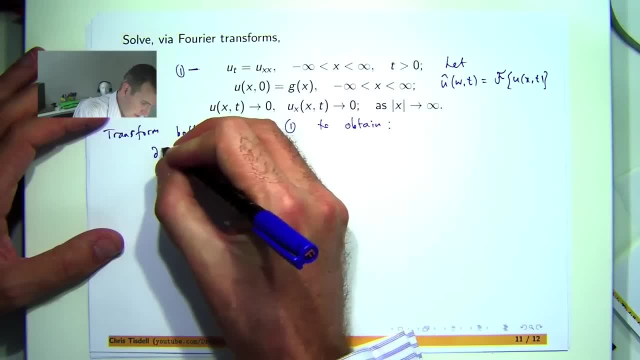 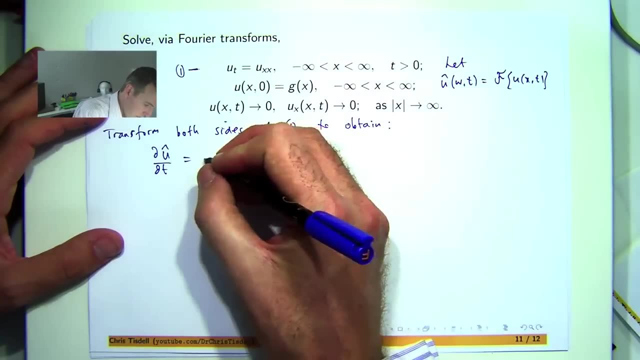 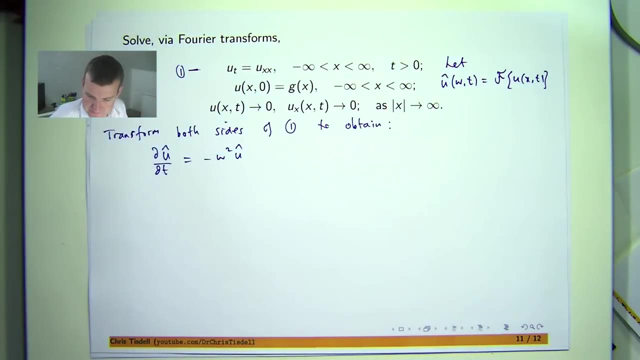 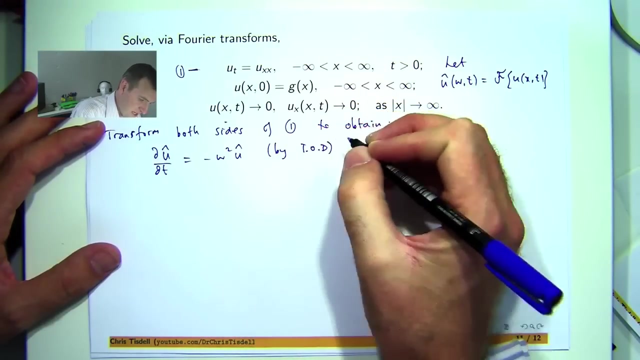 the derivative of u with respect to t, And over here, using the transform of derivatives, we'll get the following: Yes, OK. So let me just mention that we've applied TOD, or transform of derivatives, here, So now we've got a new equation, or differential equation, So we're 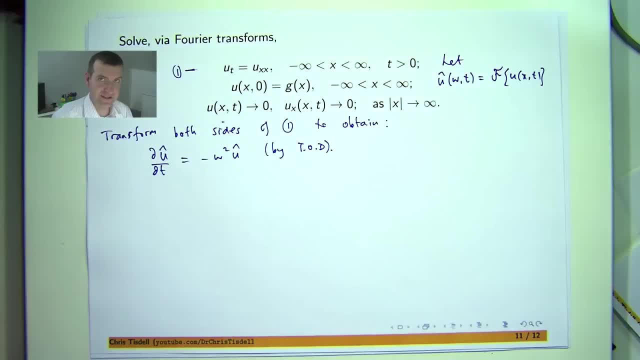 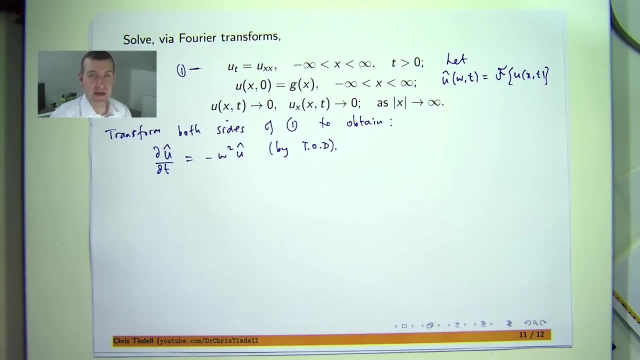 going to go back to the original equation. Notice that we've only got one partial derivative present in this differential equation. Therefore you can kind of think of it as an ordinary differential equation And, in particular, the techniques that you know for solving ordinary 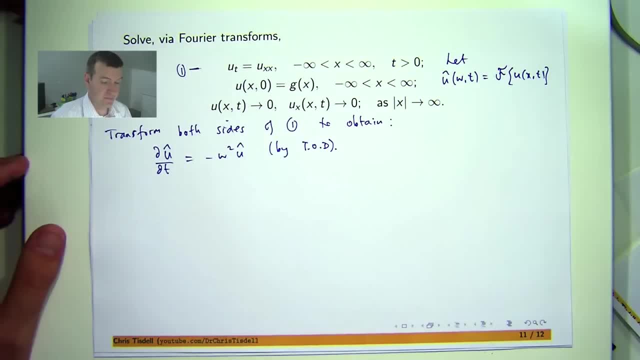 differential equations can be applied to this problem. OK, So we've transformed the problem. We're now trying to solve the transform problem. Once we've solved it, we'll try to take the inverse transform and recover the solution to our original problem. OK, This. 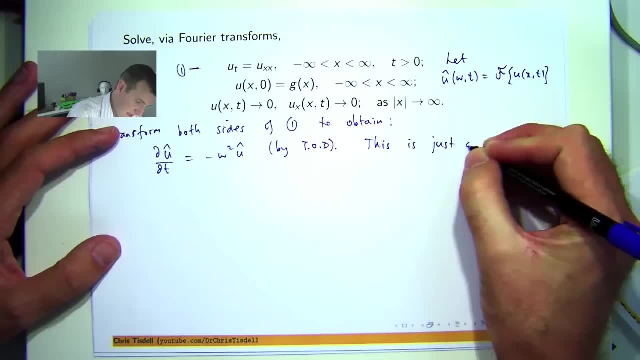 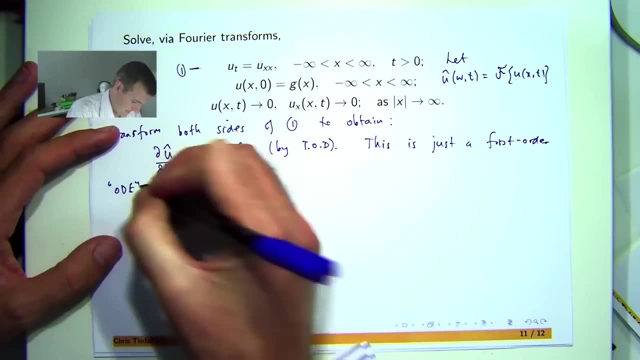 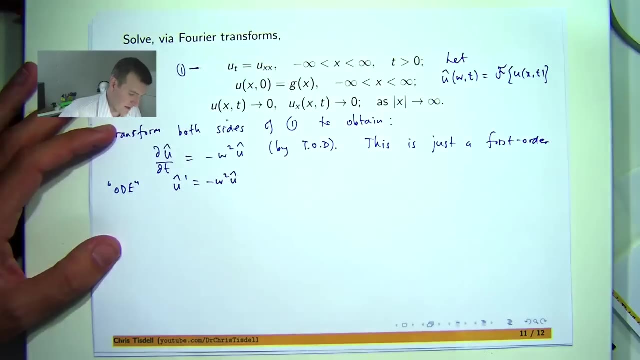 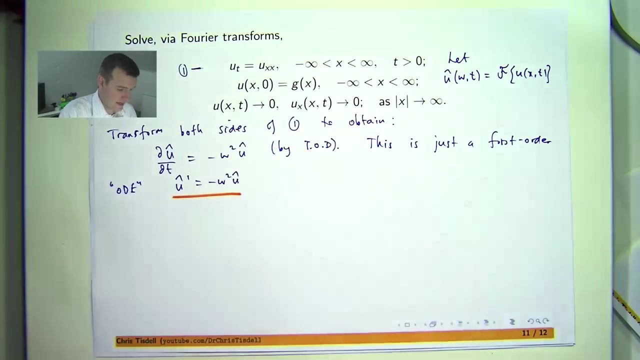 this is just a first order, ODE, OK. So I might just write it like this: OK, Where the dash means differentiation with respect to the t variable. OK, So how do we solve this? Well, in a course in calculus, or say a first course in differential equations. you're not going. 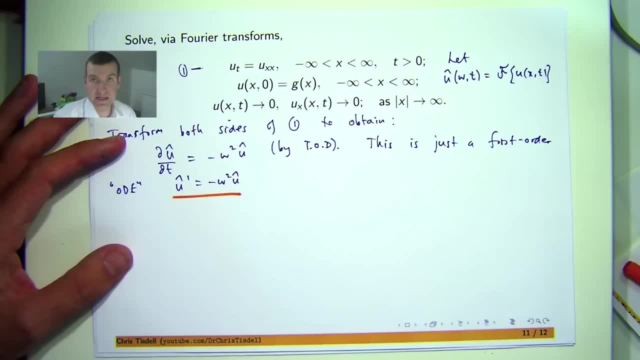 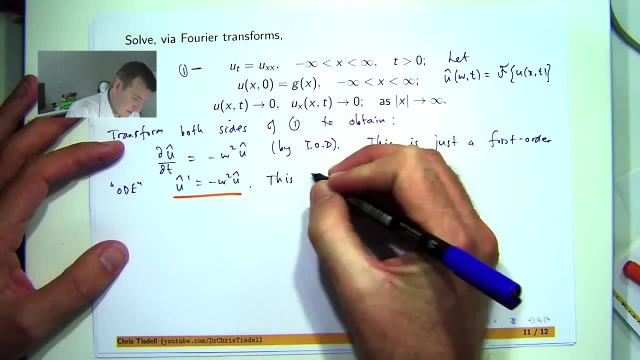 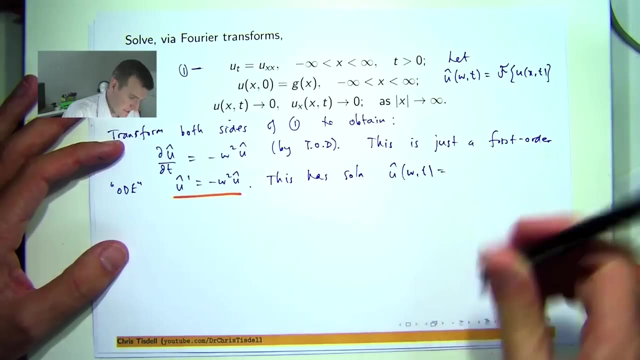 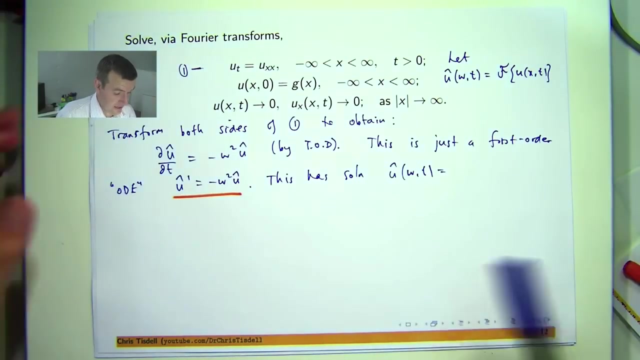 to know that the solution to this problem- treating say W as essentially playing the role of a constant- the solution is an exponential function. So this is a general solution. now It's basically e to this of e to this times, t. OK. 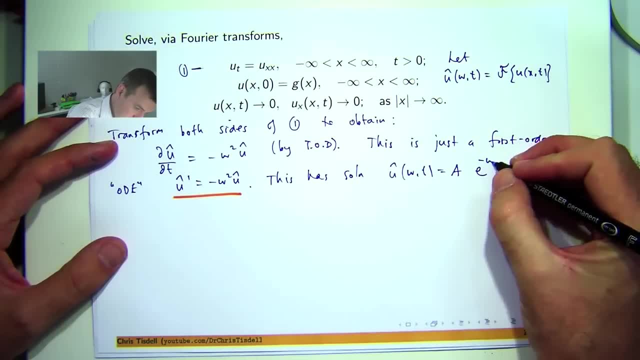 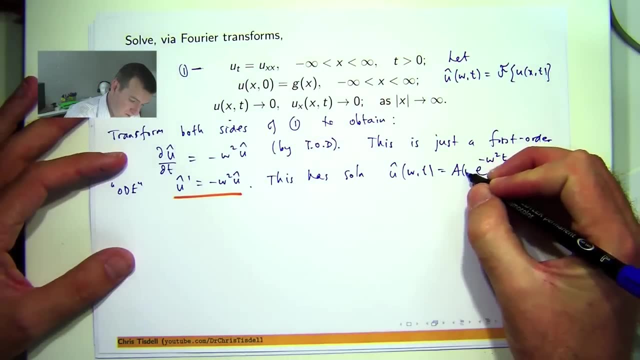 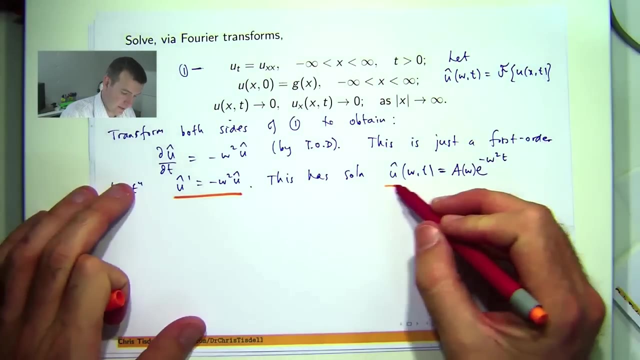 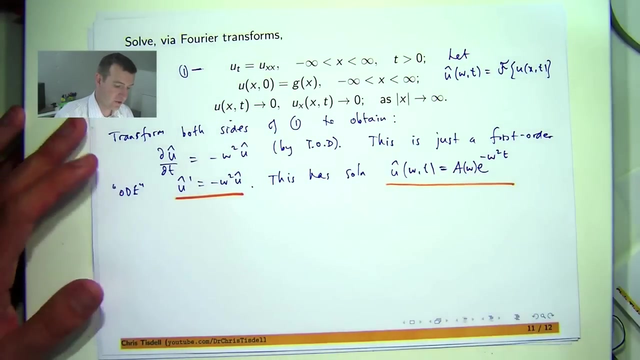 Now, you would generally put a constant here, But remember, W is a function of two variables, So this coefficient, if you like, really should be a function of W. OK, So if we can compute this function a, then we've actually solved the transform problem. So how can I compute? 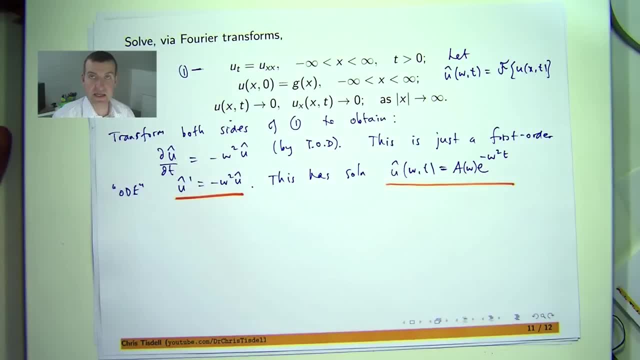 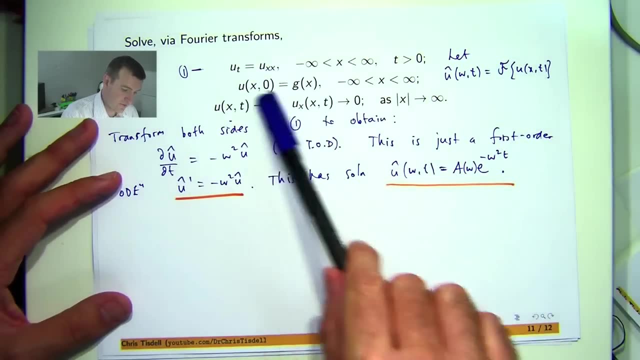 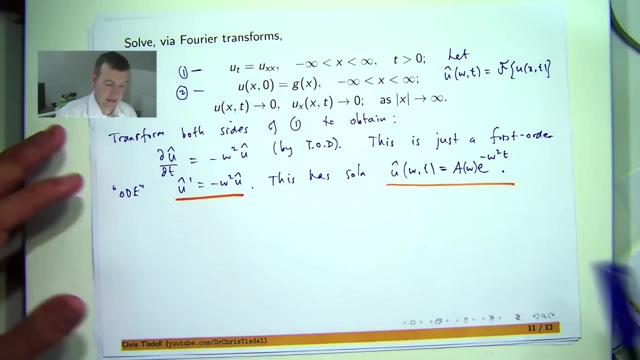 the function a. Well, let's look at the extra conditions that we're given. We're going to use the initial temperature, OK. So if we transform, say 2,, both sides of 2, we'll actually get an initial condition that is compatible with this kind of transformed general. 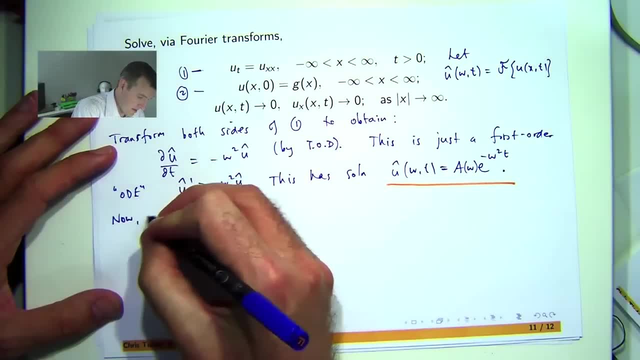 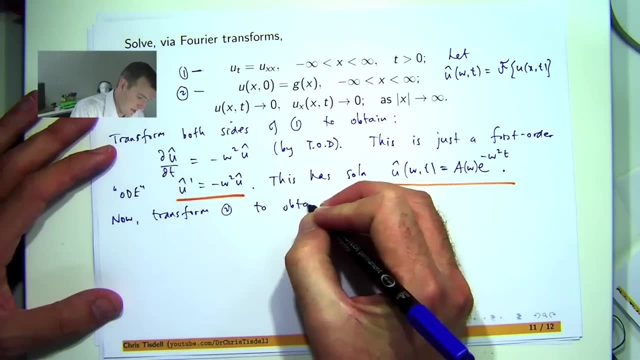 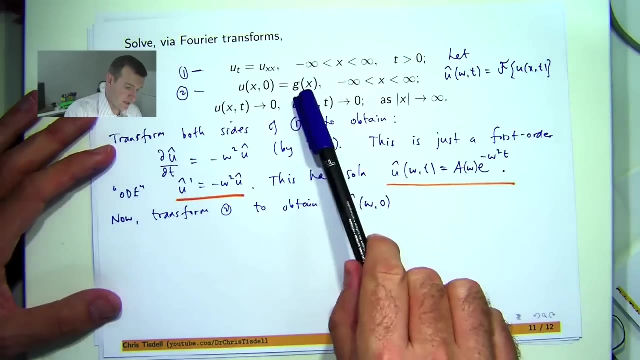 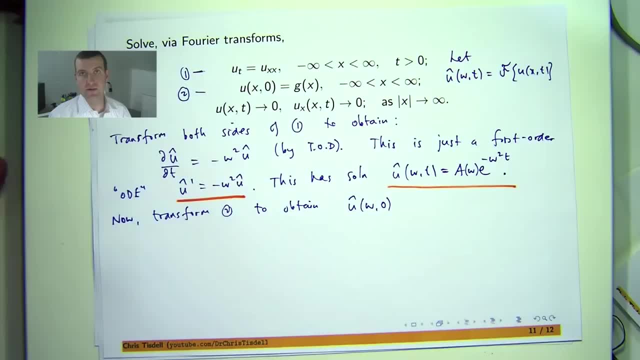 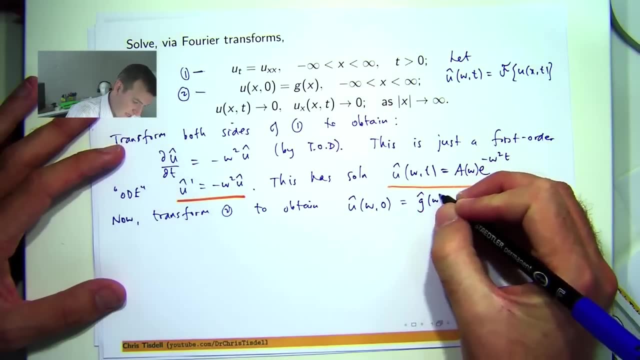 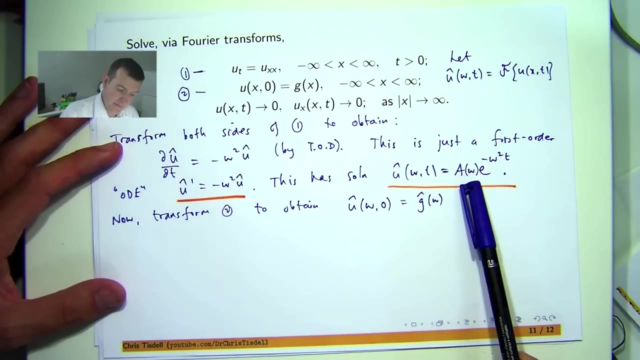 The transform of the right-hand side. well, we don't know what g is, but let's just assume it has a Fourier transform. Let's write the transform as g hat. OK, So I have this general solution. I want to refine it by computing a and I have this. 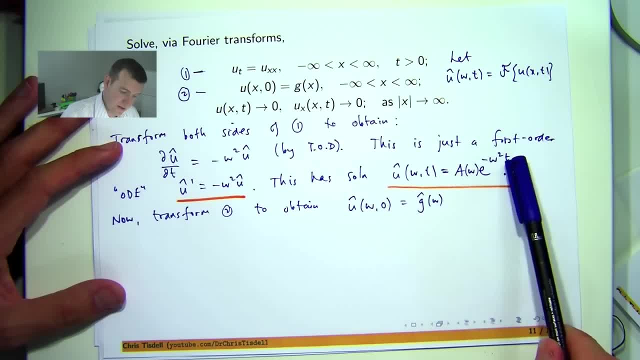 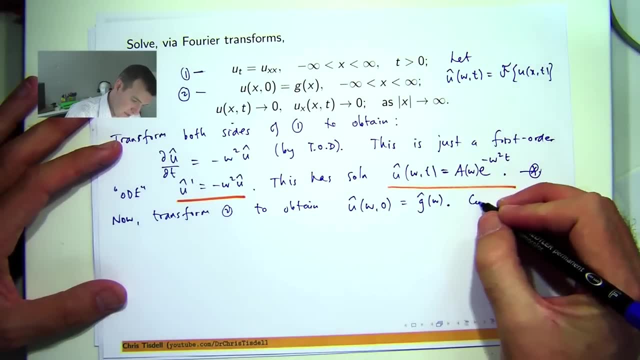 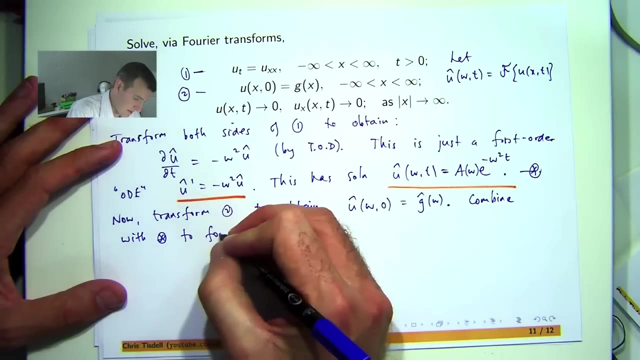 initial condition. So if I go up here and plug in: t equals 0, I know this has got to equal g hat, Okay. so let's call this star, So let's combine With star To form. okay. Well, if t equals 0, that terms going to disappear and I'll be left with a of W and that's got to equal. 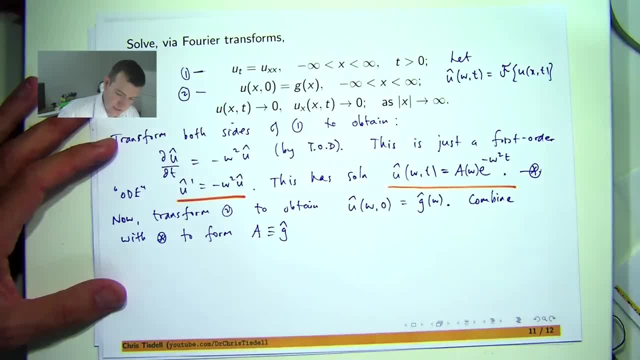 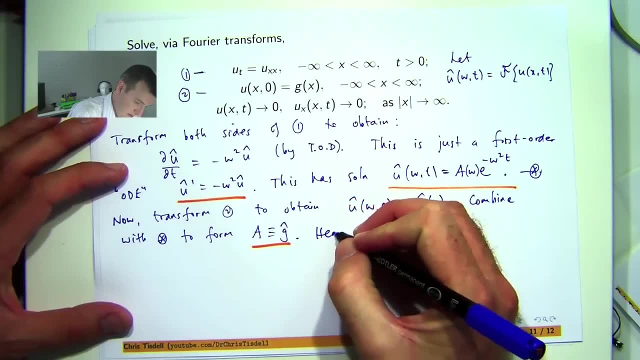 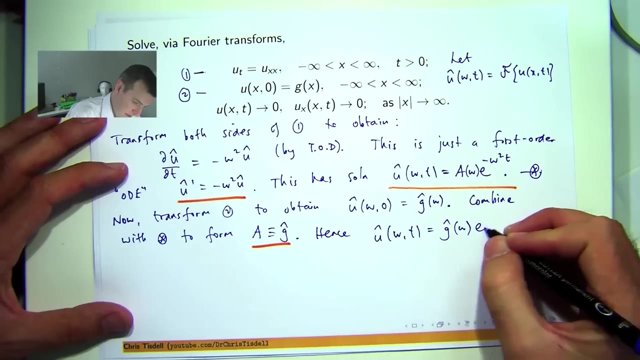 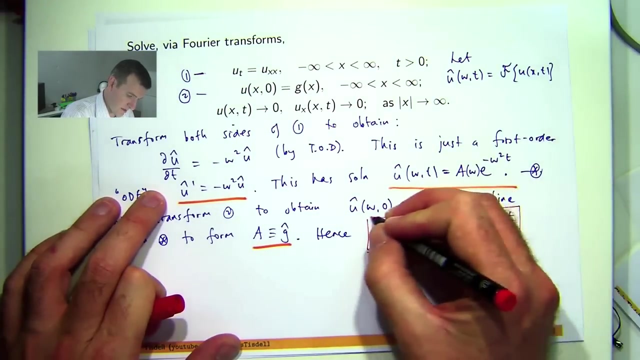 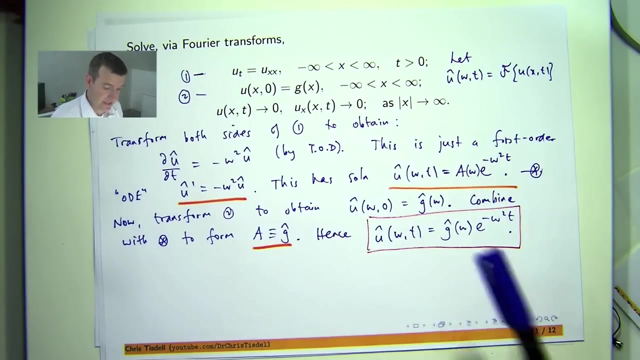 G hat. so a is identically equal to G hat. So I can now Write down my refined solution. So that is the solution to my Transform problem. So what I would like to do now is invert this or take the inverse, transform and recover U of X comma T. 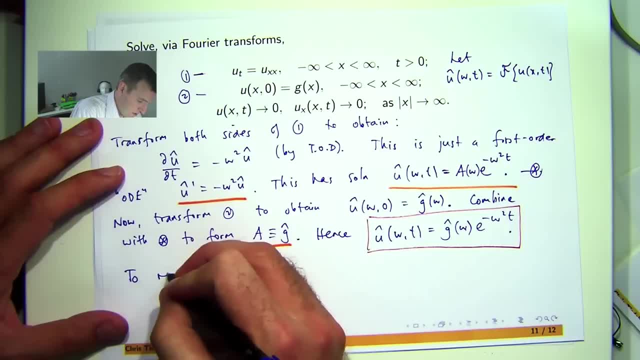 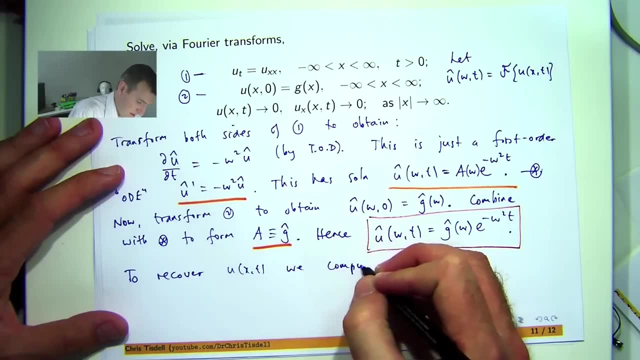 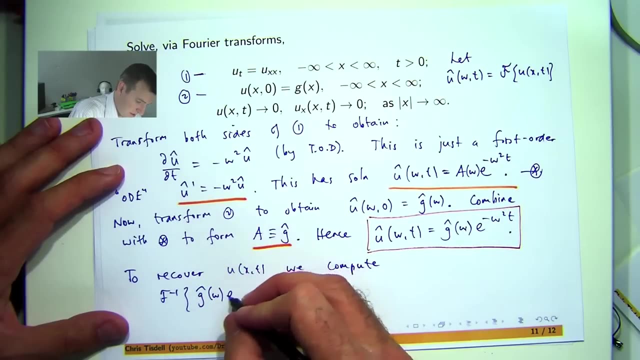 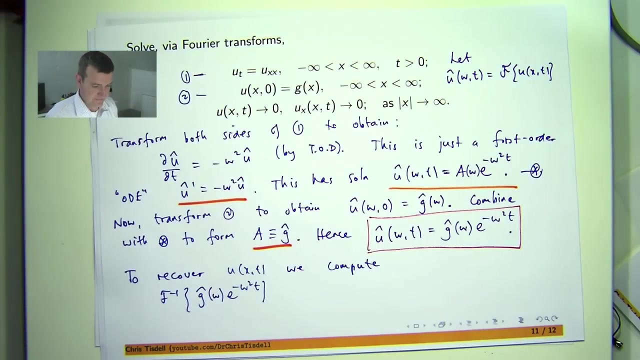 Okay, so to Recover U, We compute the inverse transform of this. Okay, so how do we do it? well, Essentially, you can see that this is a product of two functions. Okay, and in particular, this is the transform. I mean, this, essentially, is a transform of something else. 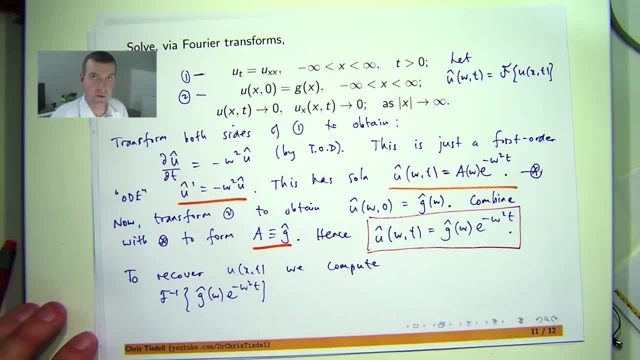 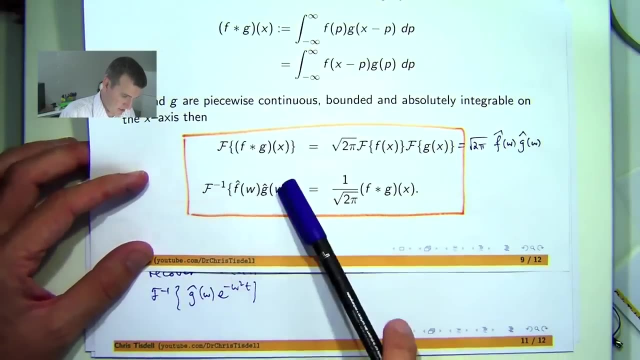 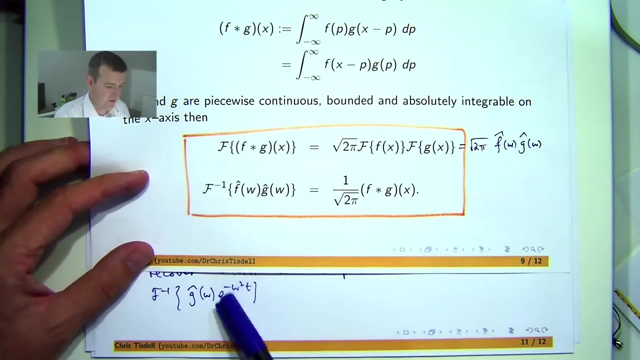 Okay, this is a bit like a Gaussian, and we know from the earlier videos That if you transform a Gaussian you get another Gaussian. Okay, so we're essentially looking at this kind of situation here, with this playing the role, say, Of f hat, of W there. obviously, this is a function of two variables. This is the function one variable. 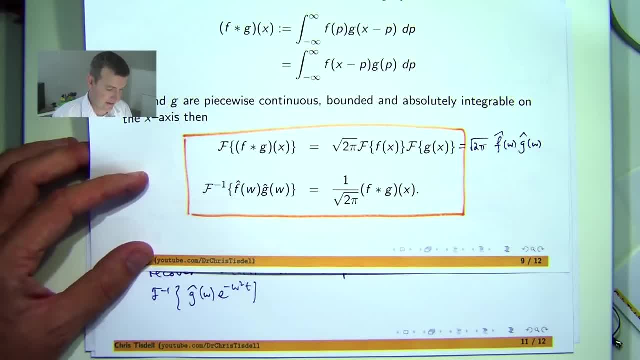 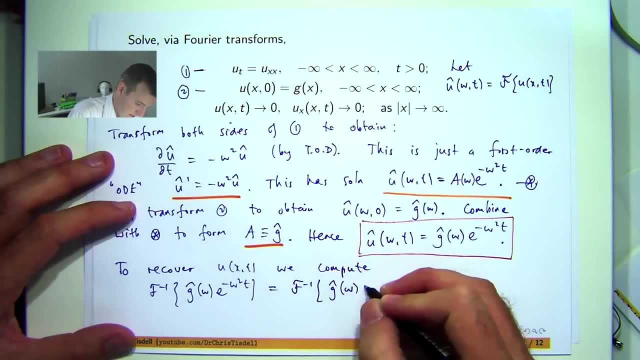 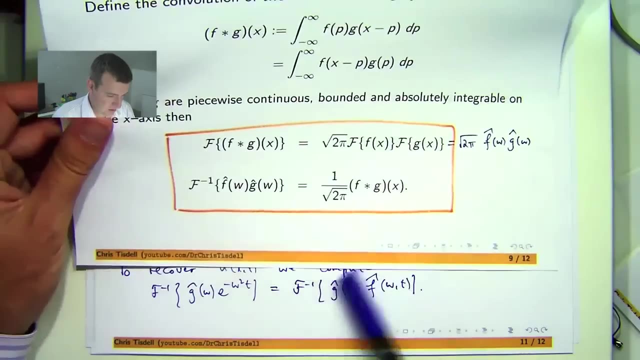 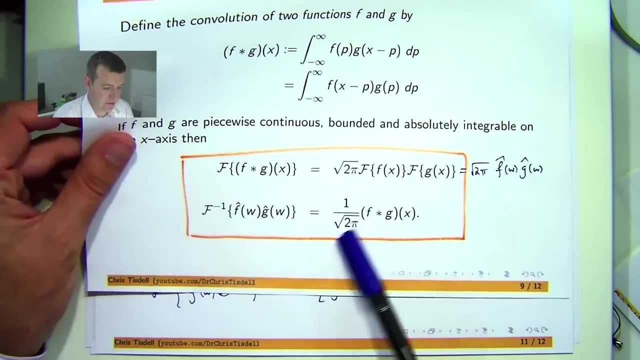 It doesn't, it doesn't matter that much. Okay, All right. so what is the solution to this? well, we compute G, we compute F, and then we take the convolution and multiply by the This is constant. that gives the inverse transform of this and which will give us our solution: you. 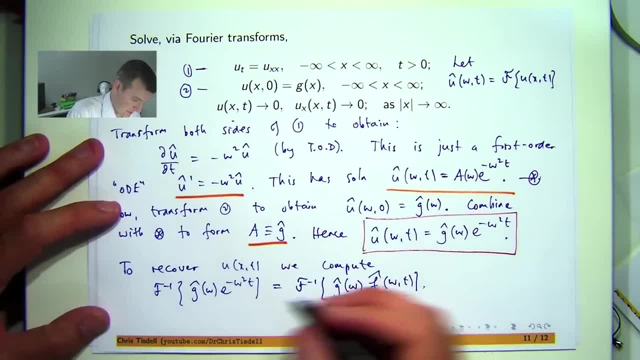 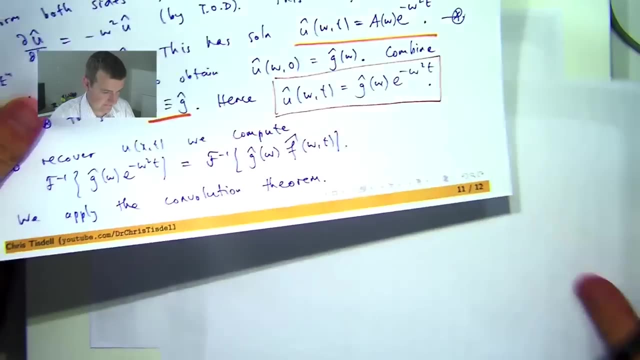 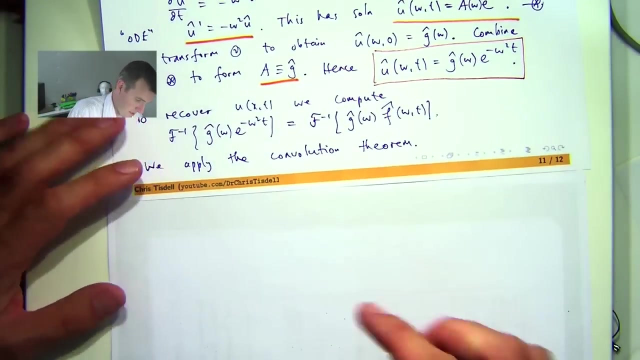 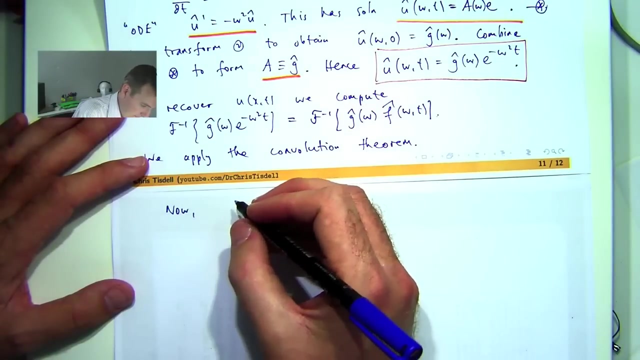 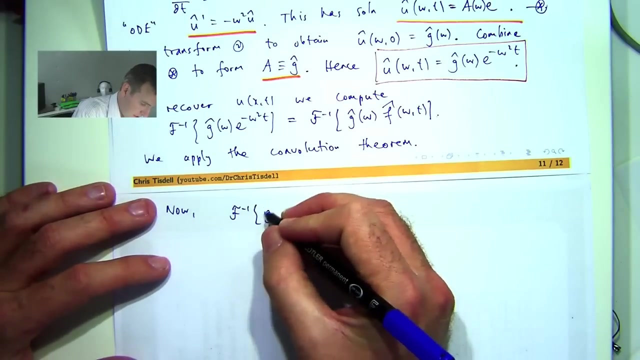 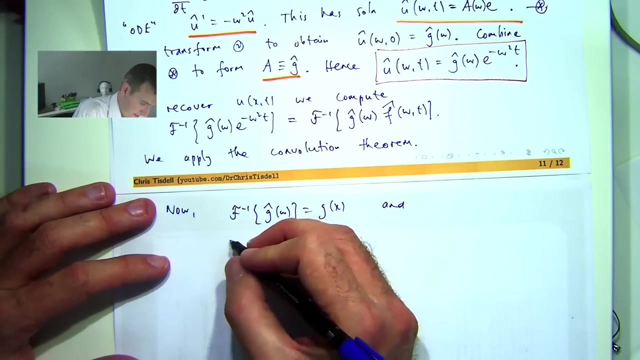 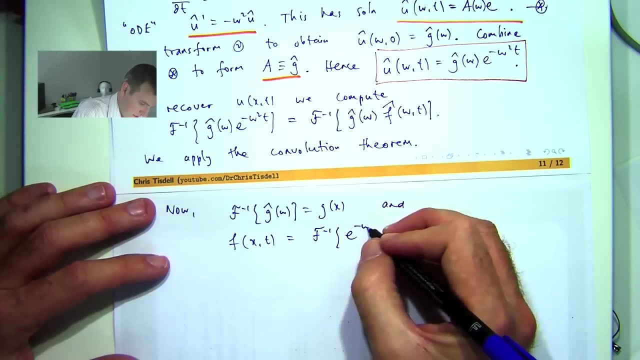 Okay, So we're going to apply the convolution theorem. All right, so how do we do that? well, Well, the inverse transform of G-hat is just G. oh Now, think of T kind of playing the role of a constant here. 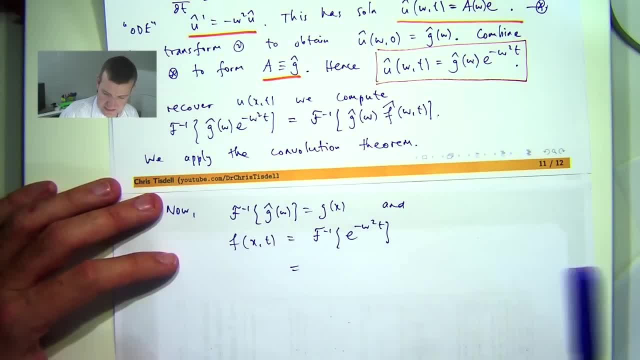 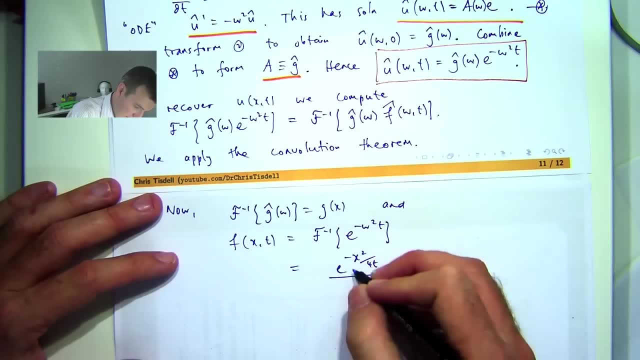 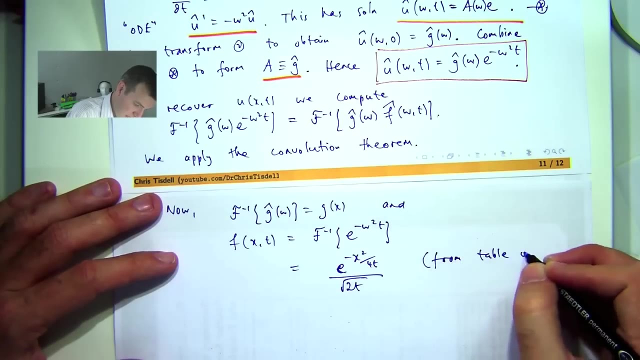 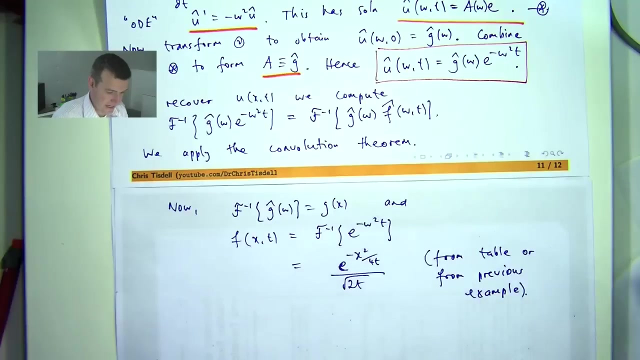 The inverse transform of this, a Gaussian is another Gaussian. okay, so you can get that from a table or from a previous example or video. okay, So what you want to do is take this and take this and calculate their convolution and then 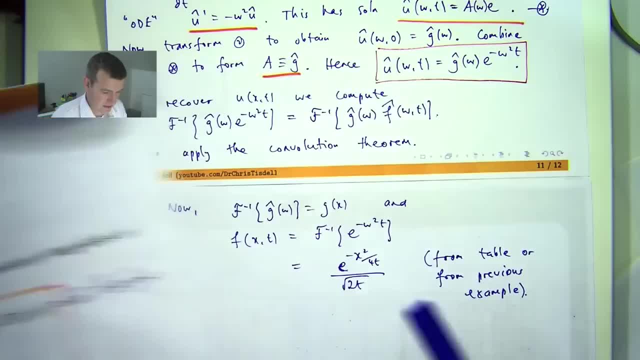 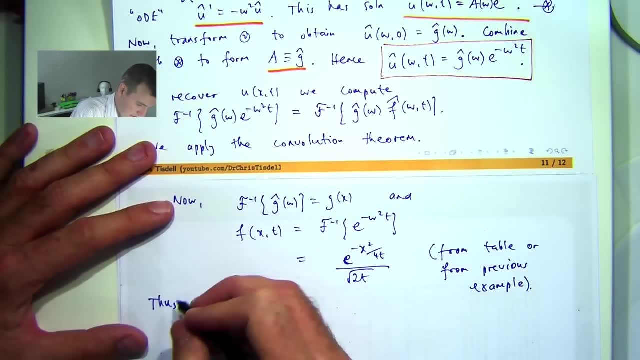 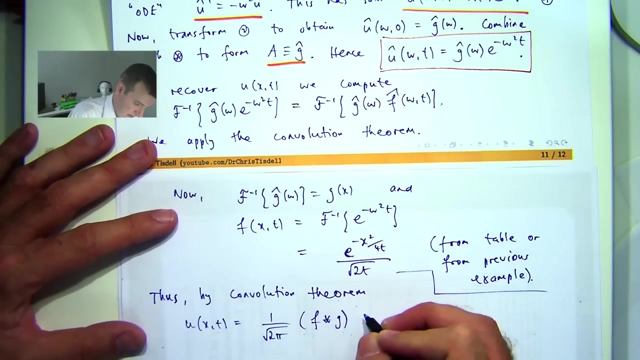 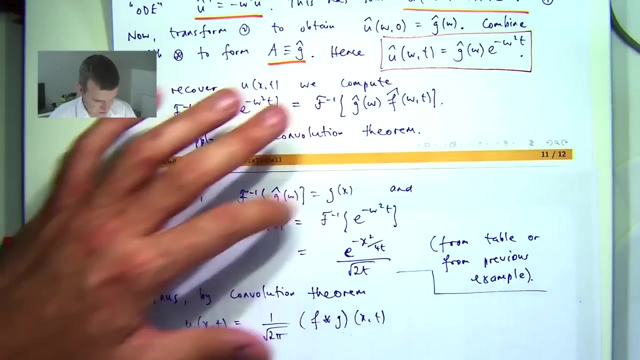 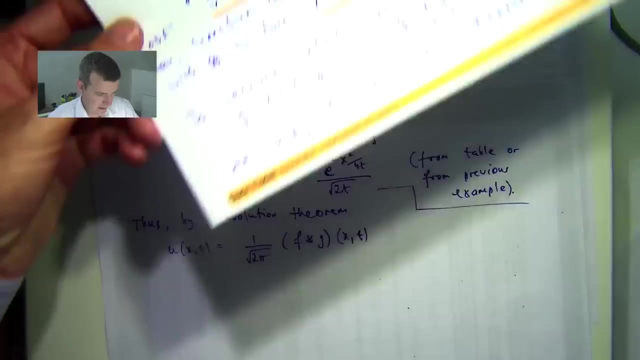 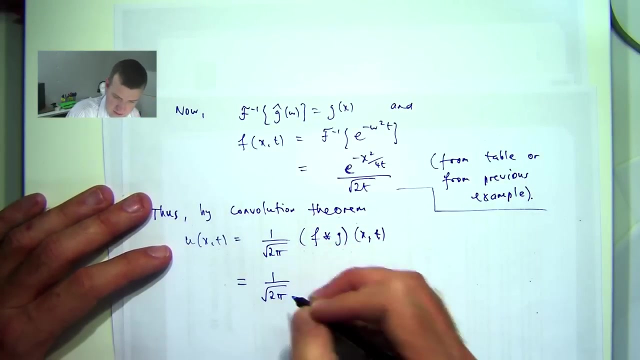 multiply through by this constant and that will give us U. okay, Okay, So it is if start. Now I'm just going to put this x comma t in to signify that you know, really, the product is a. It depends on two variables rather than one. 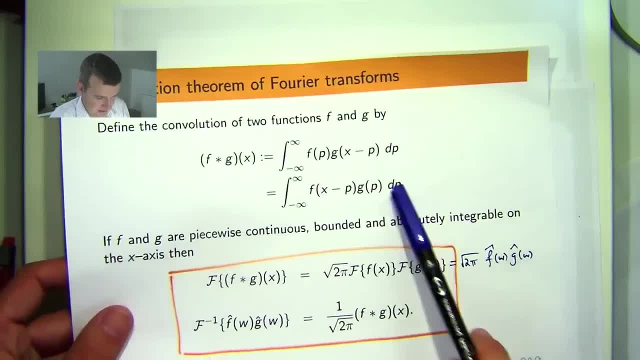 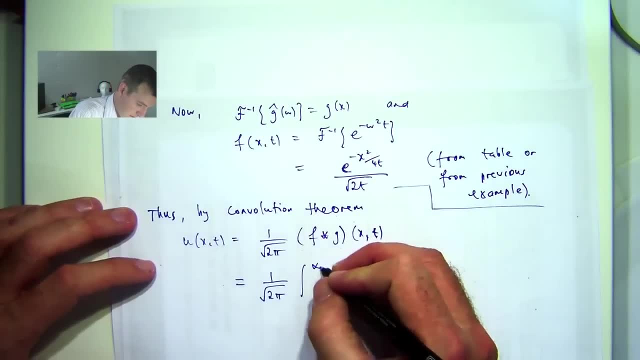 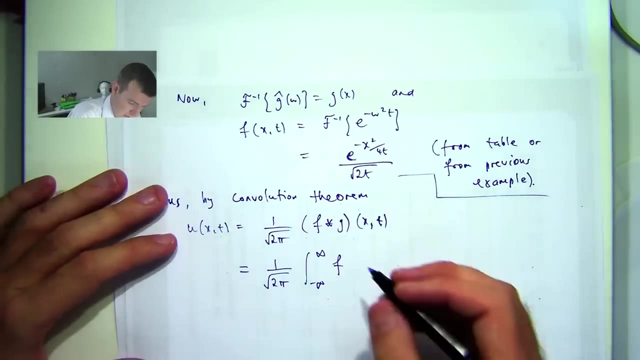 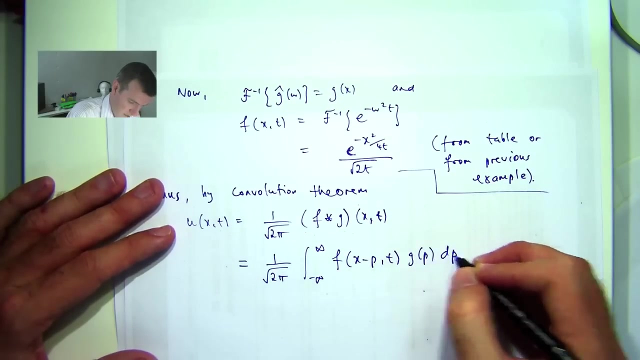 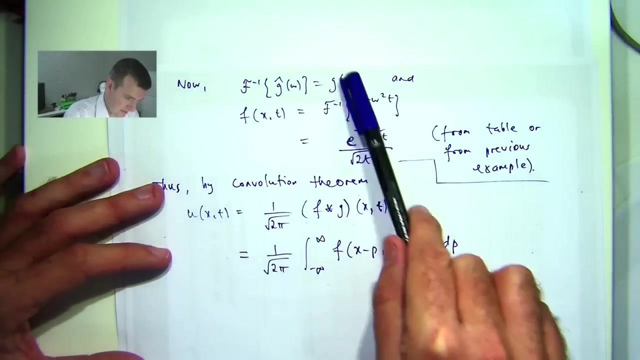 So I'm going to use this improper integral representation, And so f is that. so I replace x with x minus p in brackets, and g is up there. So I don't know what g is, so I can just write that down. 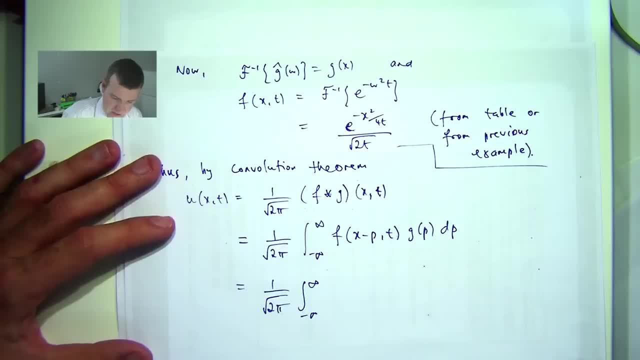 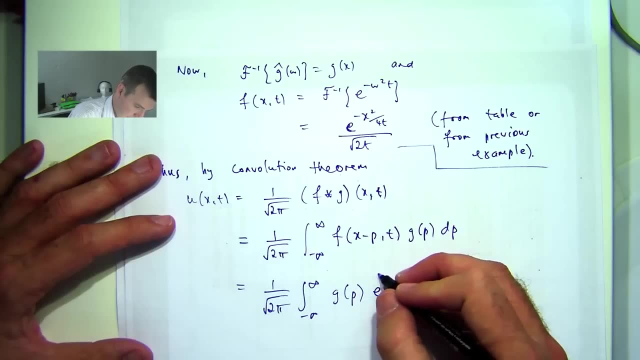 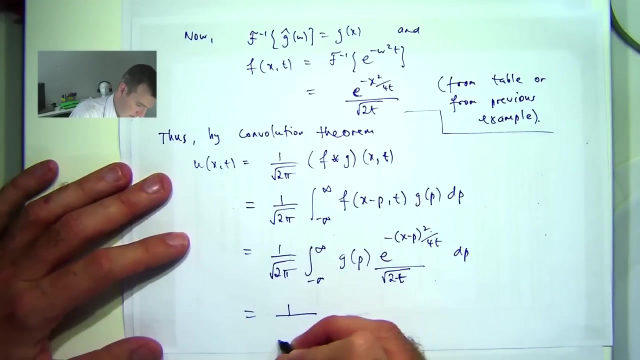 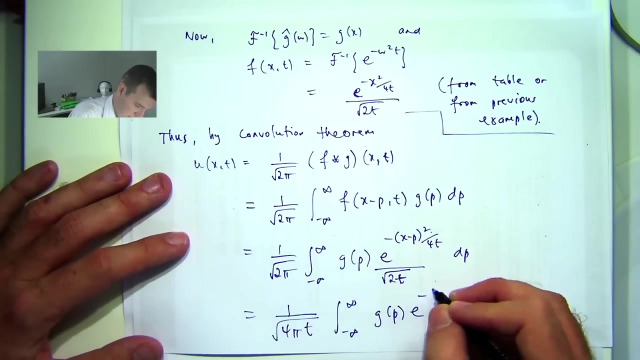 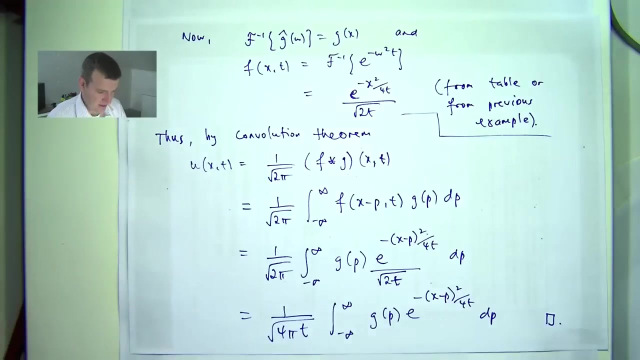 Okay, So I'm going to get something like the following: I'll just sort of switch the order around a little bit. Okay, if I take this out the front, then I get the following: Okay, So now I have my solution to my original problem. 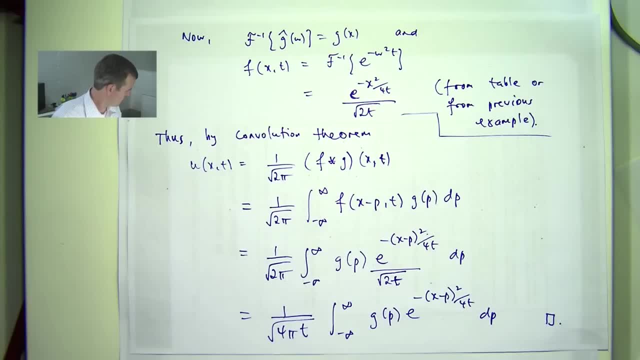 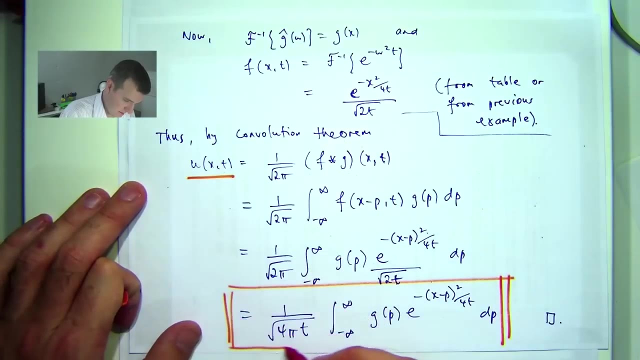 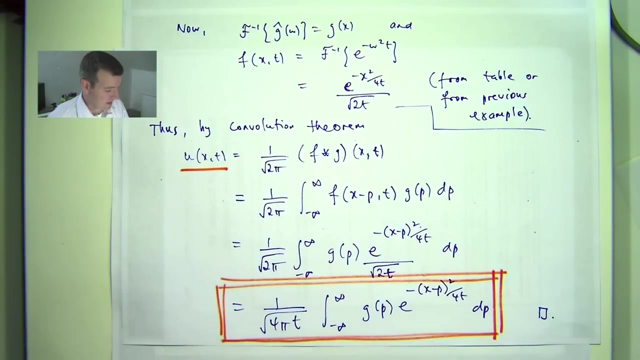 Okay, So I've now solved the problem with this form of solution. Okay, So that's it Now. in other videos, when we were studying the heat or diffusion equation, we came up with this solution by different methods. So the solution that I've shown you now some would argue that it's actually a bit more. 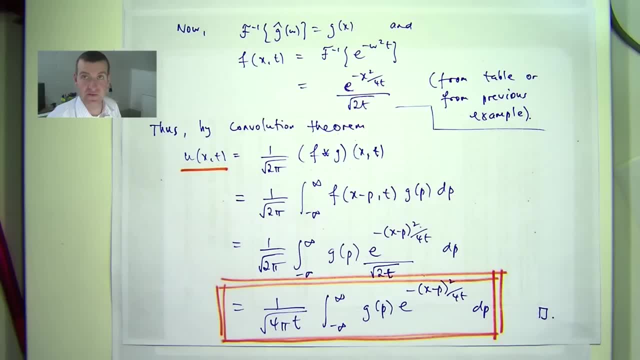 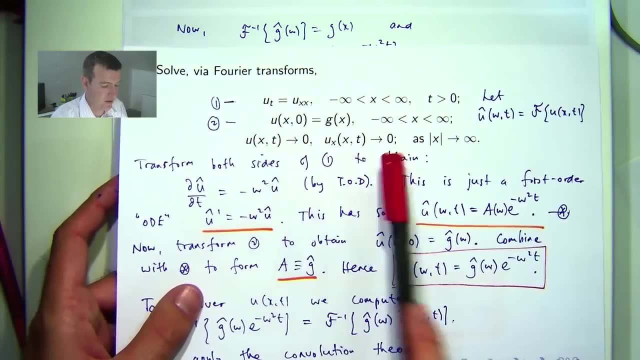 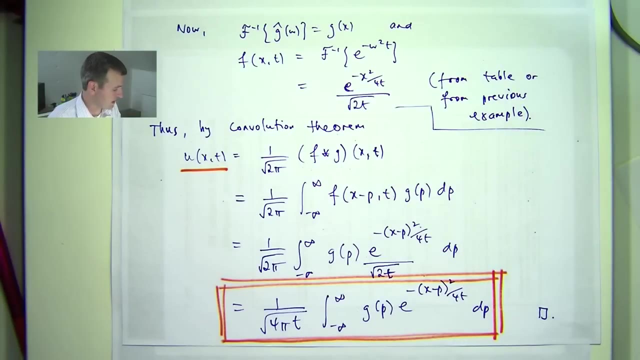 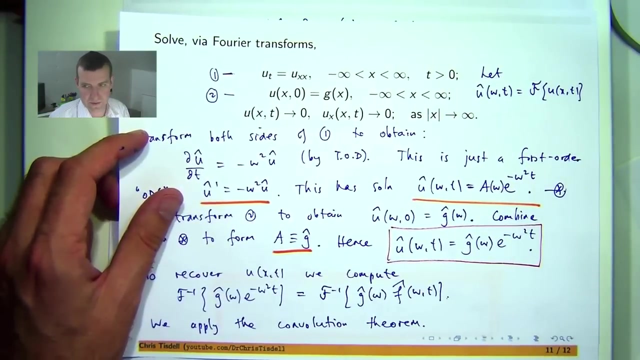 straightforward, There's less messing around, So this is one advantage of transform methods. Now, a good question here is what? Why are these two conditions here? Well, this is so that we can actually apply the transform of derivatives. They assume that basically the transforms, there's no initial or boundary conditions. 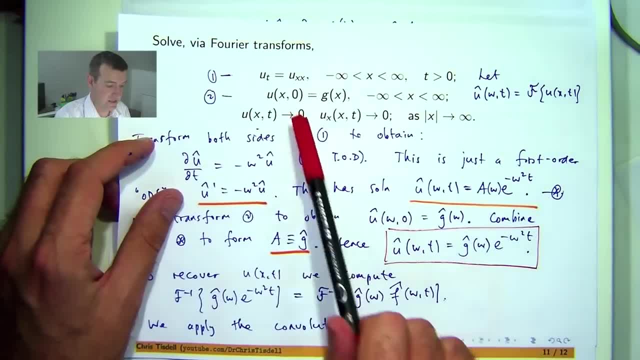 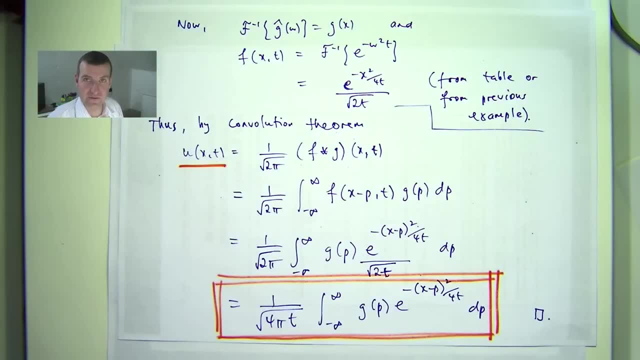 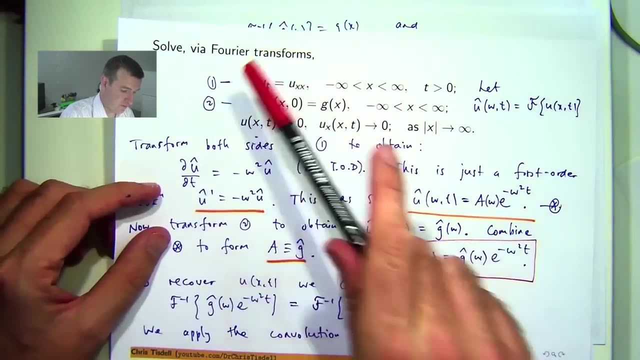 associated with the transforms of derivatives. so these things should be zero. Okay, So that is the transform method for solving the heat or diffusion equation. Again, So before, the transform methods for differential equations are usually the same. You take the problem and you transform it.